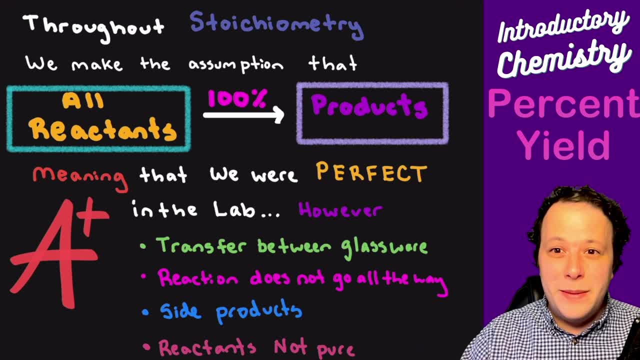 make errors because you're learning, you're trying to get your lab skills better. Sometimes reactions don't completely occur the way you want them to, but there are errors, and these are things that we have to deal with Now. where can these errors come from? Well, the first thing we want to do is to 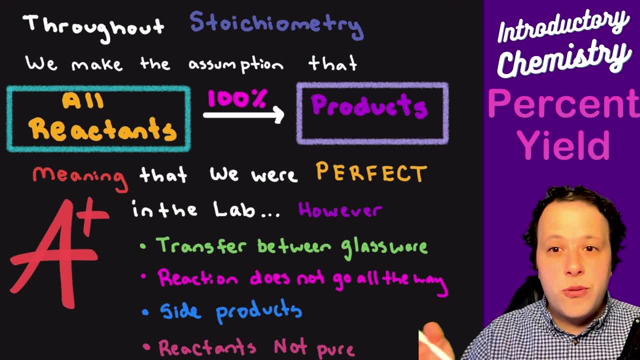 calculate the number of errors that we make in the lab. So what we're going to do is we're going to calculate the number of errors that we make in the lab. So what we're going to do is we're going to: Alright, alright, Let's see. So I'm going to do a little test field test here. So initially, you 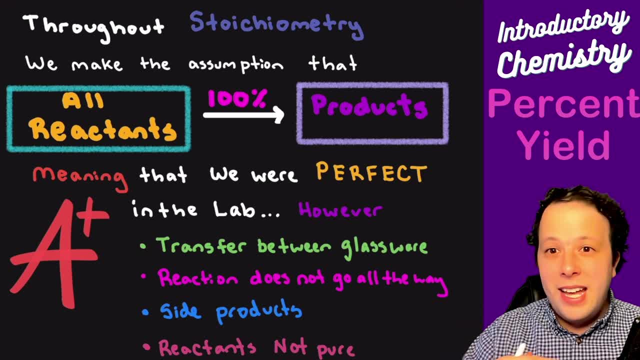 need to calculate the level of errors that we're going to solve Now when we do these exams on small hospitals. we expect to go up by 10 or so. I don't think itloe at all, but to be honest with 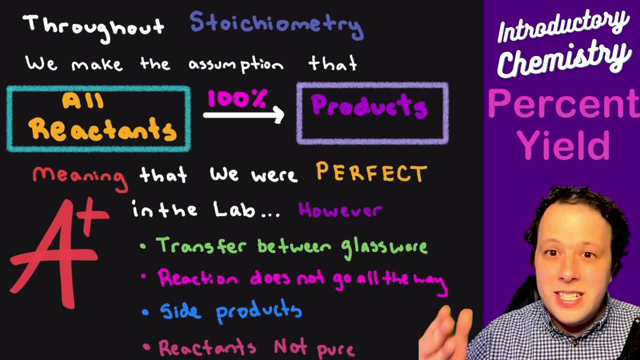 you. it's a rebuke. You need to buy it, but I don't have a lot of money to buy it, so we'll end it that way for now. The first thing is how you start to calculate the level of errors. So 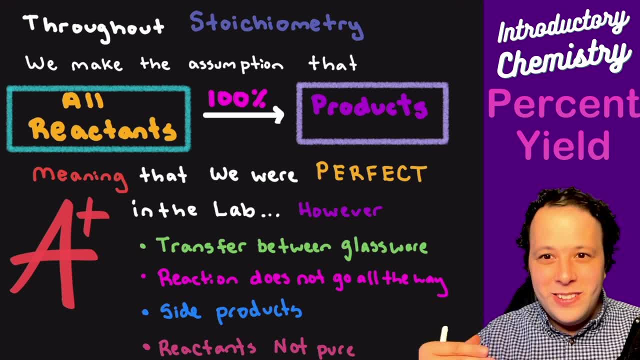 this is roughly. if you are able apply the speeds like this, or you want to recall all the values that we handle, how and when we're competent to make err, Okay. so, for example, here's what that could be made: is maybe you made a side product, meaning that another reaction occurred. 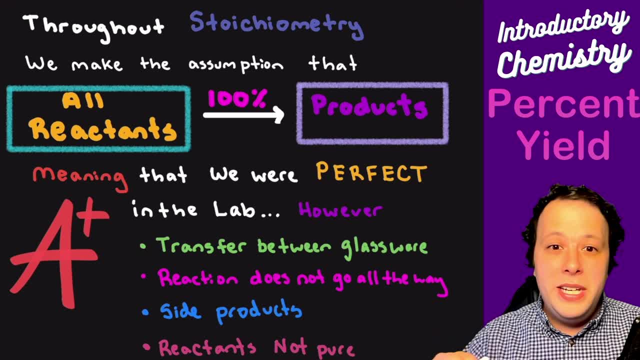 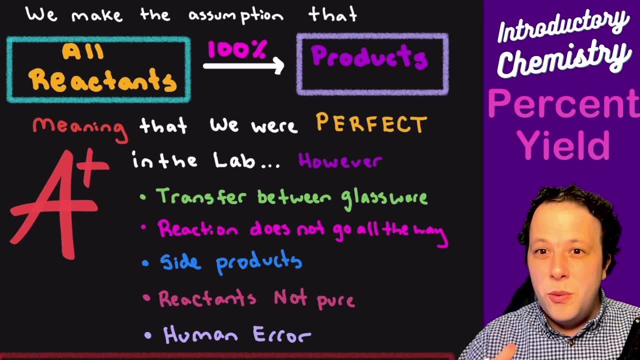 without your knowledge, or the reactant isn't p, or let's say the reactants weren't even pure to begin with. so let's say, if you just had, like some, maybe not the best quality ingredients, well then yeah, you're gonna have different, different uh products in the very end, or just human error to begin with. 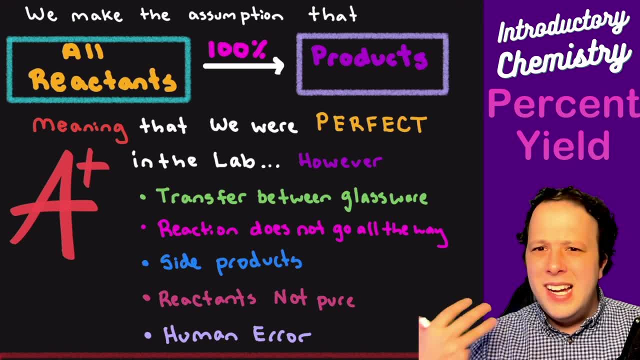 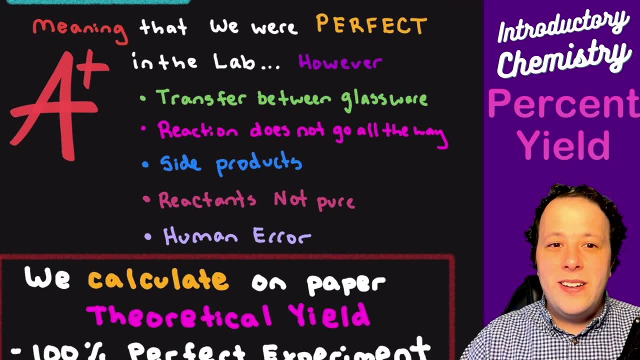 maybe you just made a mistake or forgot to do something, or added too much water, or whatever it is. there are going to be errors. so when we are calculating this, we calculate on paper- the theoretical yield, which is something that you've been doing all along. this is all stoichiometry. 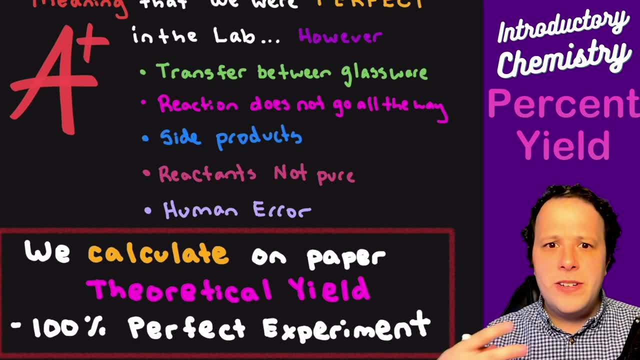 calculations. so, whether it's mass to mass, gas, stoichiometry, solution stoichiometry, you're assuming that you have a perfect experiment right. this is all about mass conservation and being perfect, and that is a true law. however, we do make errors and there is mass that can be lost. 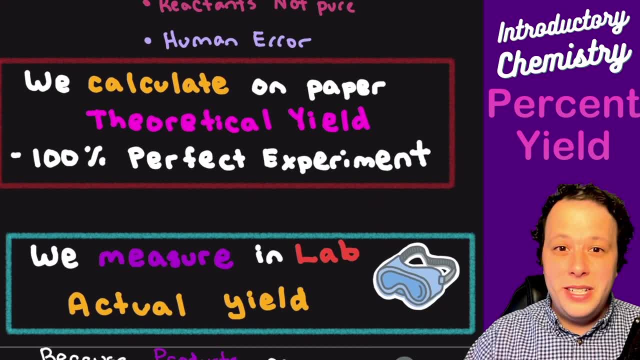 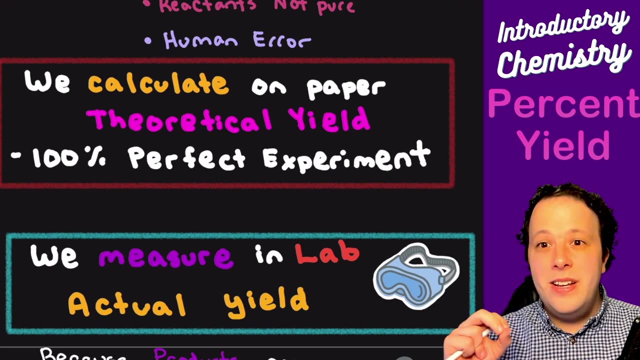 so if something is lost, this is what the actual yield is and what we measure in lab. so we compare the two numbers to see: well, how good did you do when you were in the lab? it gives us a reference point to see: can we improve right? one of the things about school is all about improvement and getting 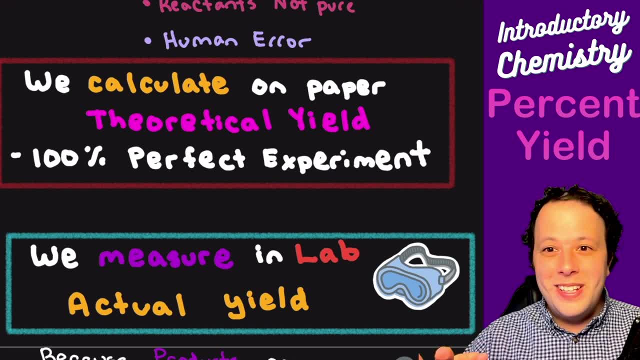 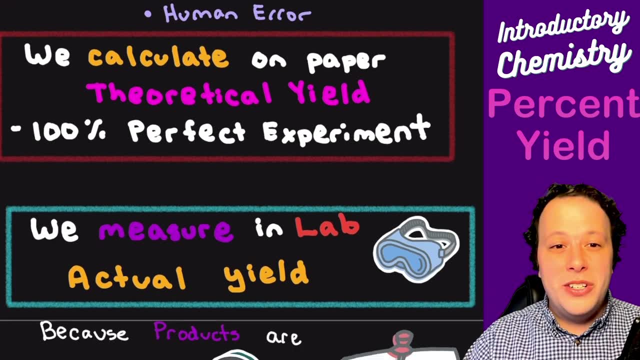 better, right, if you were getting 100 on everything going throughout the gate? then you don't need to be in school, right? you can just start working in the field that you want to be in. but we do this because we want to learn, we want to grow. 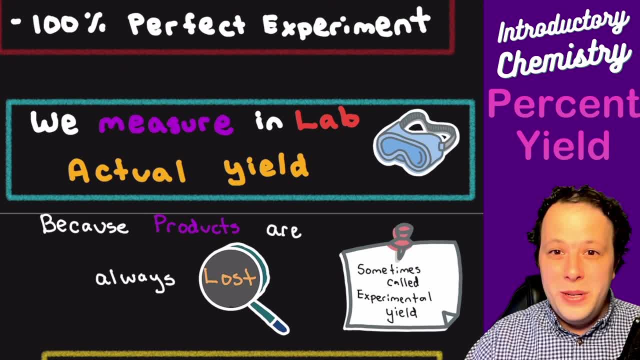 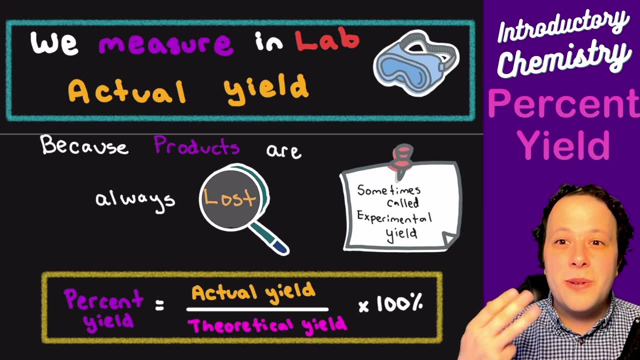 and the whole idea here is when it comes to chemistry- is, products are always lost. we're always trying to search for them with our little magnifying glass, but we always are losing a little bit. so we're going to be using this formula to help us try to understand this. 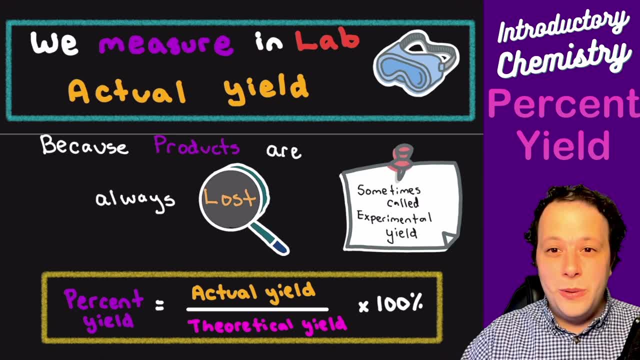 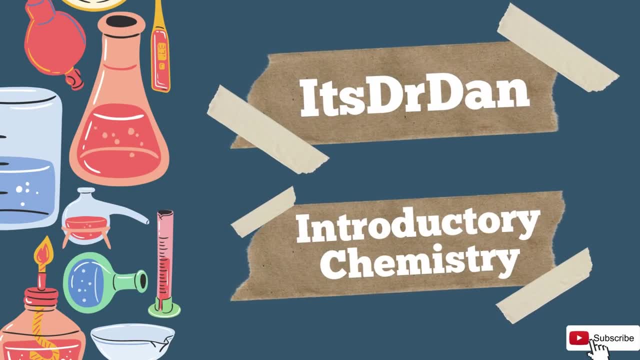 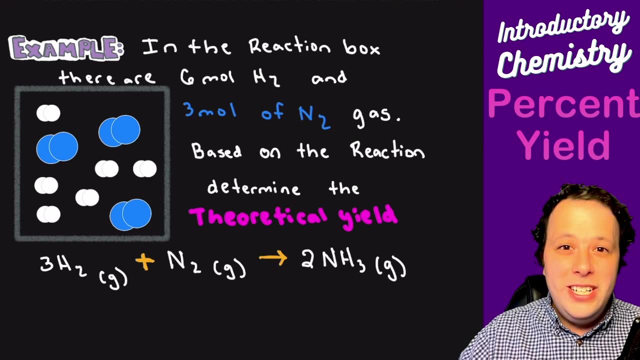 so let's try to take a look at an example of how this could work, and then we'll get into some harder stoichiometry. examples. in the reaction box there are six moles of hydrogen gas and three moles of nitrogen gas. based on the reaction determine the theoretical yield based 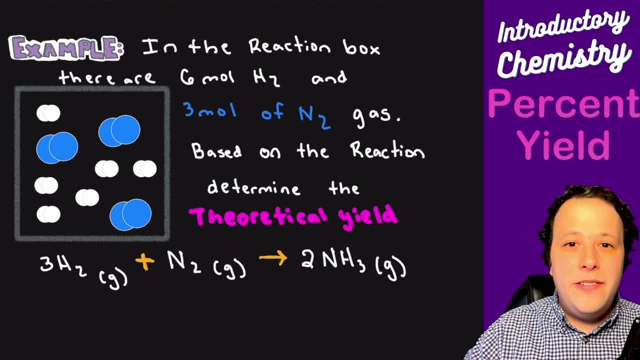 on the following chemical expression: well, if we were doing this and we wanted to figure out exactly how much ammonia you were going to make, which is your theoretical yield, what would we do? well, the first thing is that we saw is that we had six moles of h2. so if we wanted to convert, 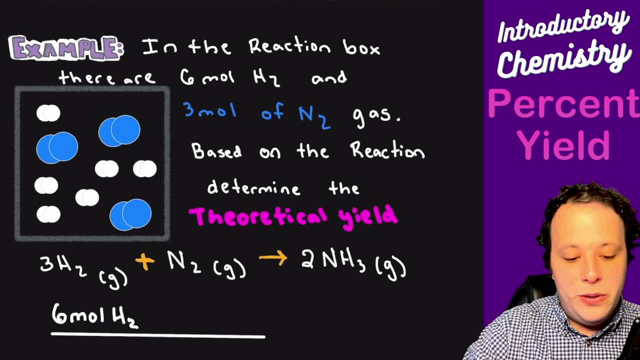 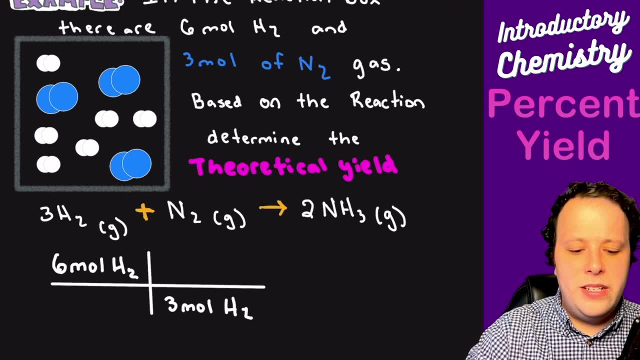 that using this formula. well, we would just use our molar coefficients and we can see that, okay, for three moles of h2, we are going to be making two moles of ammonia. so if we were to do this little conversion here, we are going to quickly see that we would obtain four moles of ammonia that are: 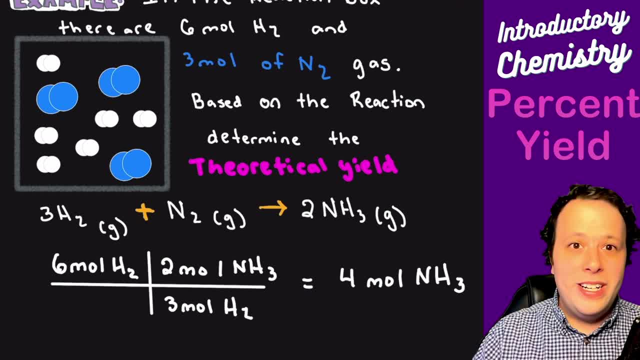 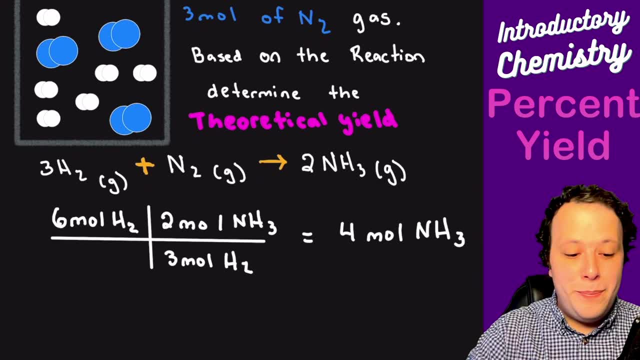 possible. now the thing is that this is a limiting reagent problem because you were given two different starting points. we were also told: hey, we have three moles of nitrogen in that box two, and we can see it as well. there are these little, the little, uh, blue orbs that are here. 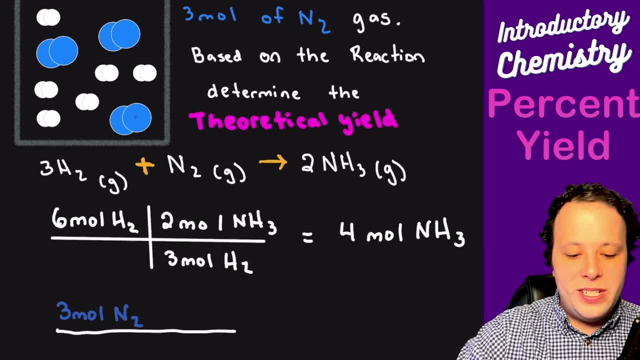 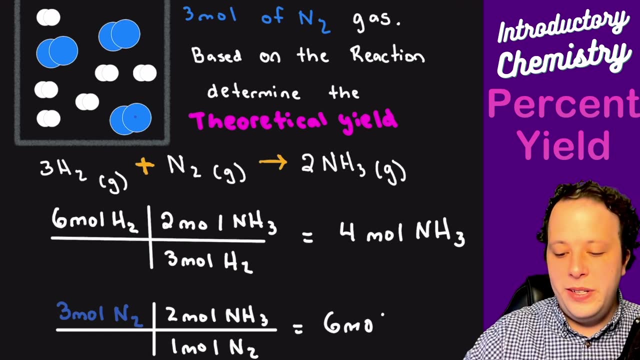 um are reacting as well. so if i have three moles of nitrogen and from our chemical equation we can see that one mole of nitrogen reacts and it creates two moles of ammonia, well, this is going to make a total of six moles of ammonia. well, which one is the theoretical yield? well, it's all about. 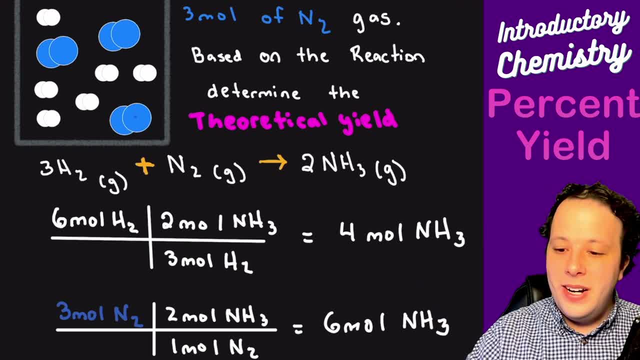 which made less out of the two. so our answer in this case is going to be that hydrogen was the and our possible theoretical yield is going to be- uh, going to be hydrogen in this case, making only four moles of ammonia. okay, so our theoretical yield is four. 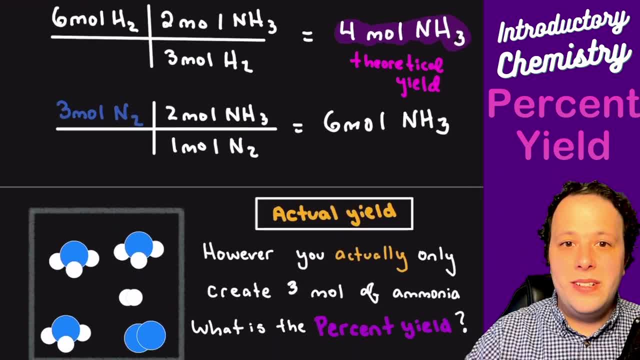 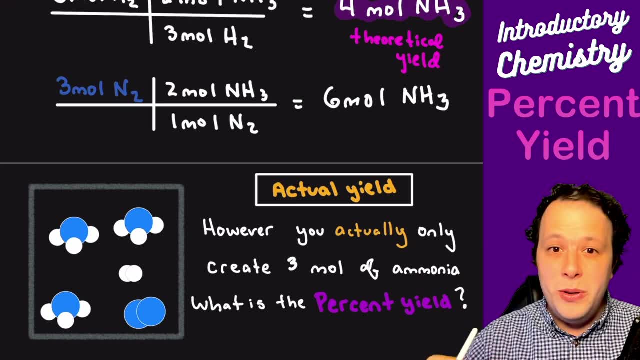 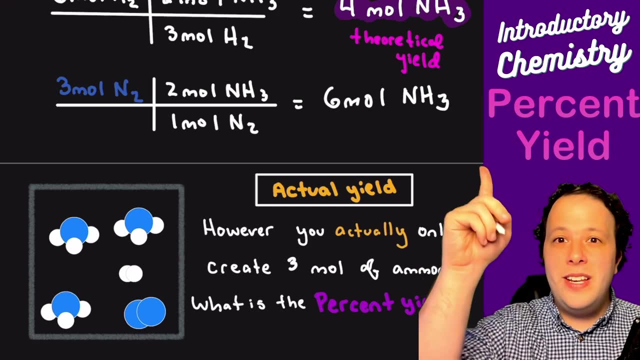 now, if we wanted to calculate, let's say, percent yield, how exactly would you do this? well, so let's say: if, however, you actually only created three moles of ammonia in the lab, what is your percent yield? well, so this is your actual, which is three. your theoretical was four. so what do you got to do? 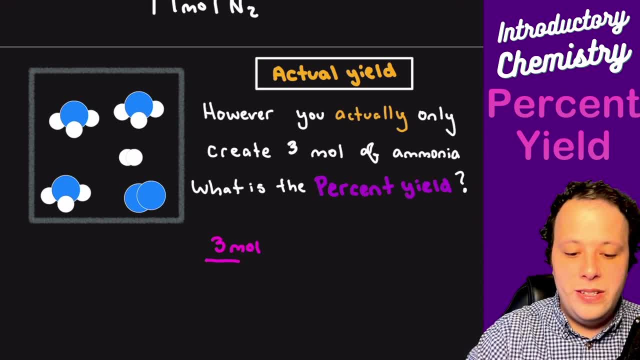 is, you'll take three moles, which is your actual yield. divide that by four moles, which was our theoretical. we calculated that together, so telling us that you have about a 75 percent yield within your reaction, which is pretty good actually, in chemistry to get about 75 yield a lot of times. 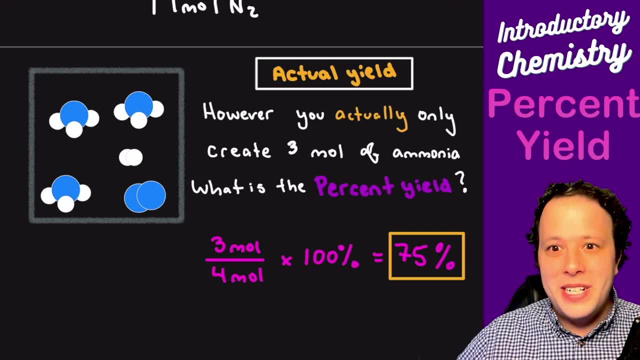 when you're doing organic chemistry. you might be lucky if you even get five or ten percent yield, depending on what reaction you were trying to do. so that's the basic idea. how much were you supposed to make and how much did you actually make when you did the experiment? all right, let's take a look. 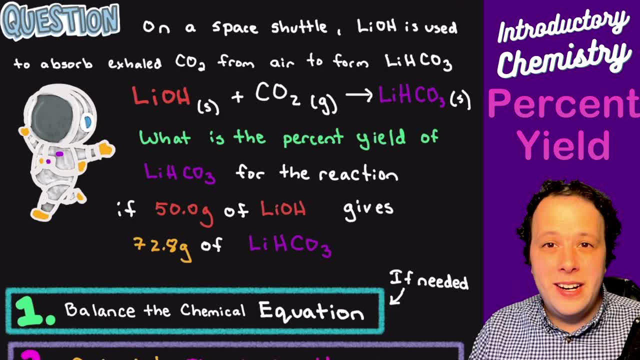 at some different stoichiometry examples from the air to form lithium bicarbonate. so lithium hydroxide plus co2 makes lithium bicarbonate or lithium hydrogen carbonate. what is the percent yield of lithium bicarbonate for the reaction if 50 grams of lithium hydroxide 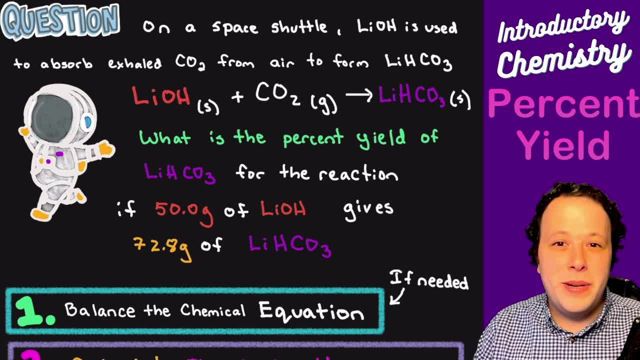 gives 72.8 grams of lithium bicarbonate. so the first thing is that what a lot of students will do is they want to just divide these two numbers and then times it by 100 and think they are done. the thing is that would be very, very wrong. we can't just take 50 grams and divide it by 72.8. 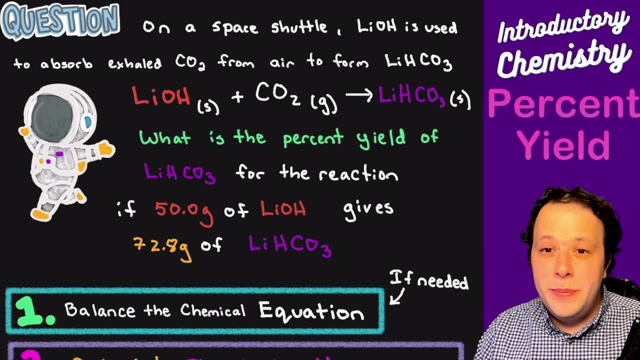 and be done with the problem. we need to convert it to be the same molecule when we are comparing the two numbers. so we need to do the stoichiometry for 50 grams of lithium hydroxide and then convert it to lithium bicarbonate, so in 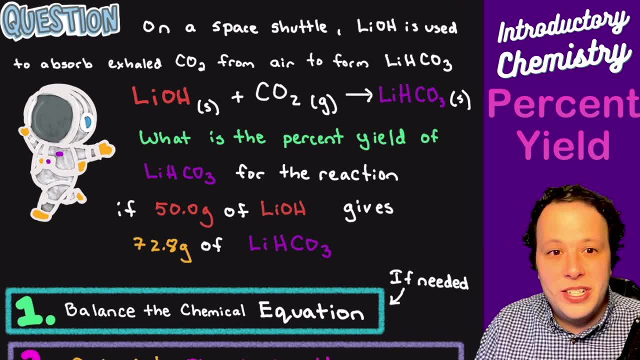 this case using mass stoichiometry to do the conversion. so now, whenever we do these, we always need to check if, if the chemical equation is balanced. typically, the easiest way to know if it is is if you see coefficients. but with this one there are no coefficients. but you can, you might. 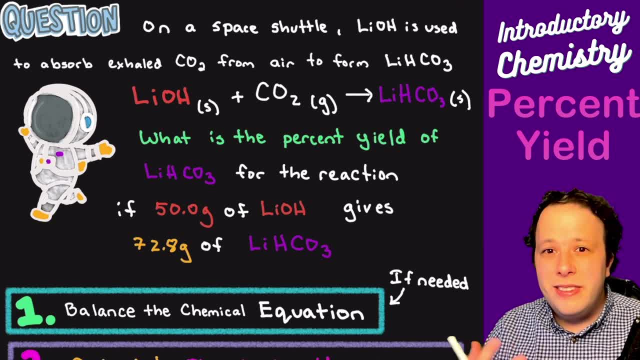 be able to quickly identify that it is balanced. you have one lithium on each side, one carbon and then three oxygens, so it's pretty quick to see that that this one is balanced. so we don't have to do anything else. so what we are going to do is we need to calculate what the theoretical yield. 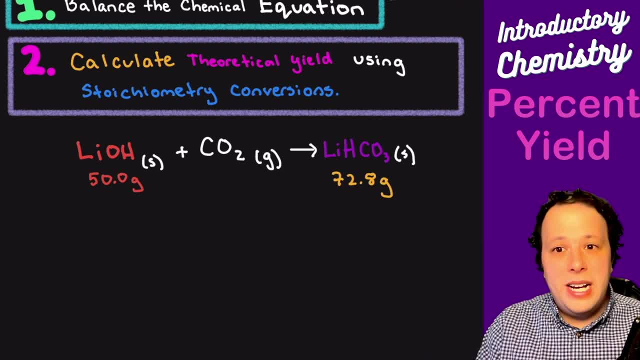 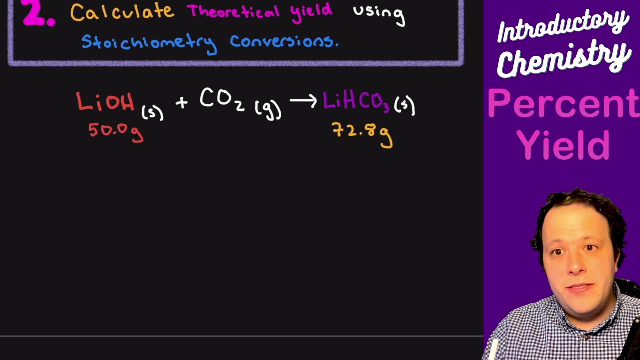 is using stoichiometry conversions, so we want to write down all the important pieces of information that we were given, which was 50 grams of lithium hydroxide, and then what our actual yield was, which was 72.8. keep in mind: whenever there's actual yields involved, it's always generally given to you in. 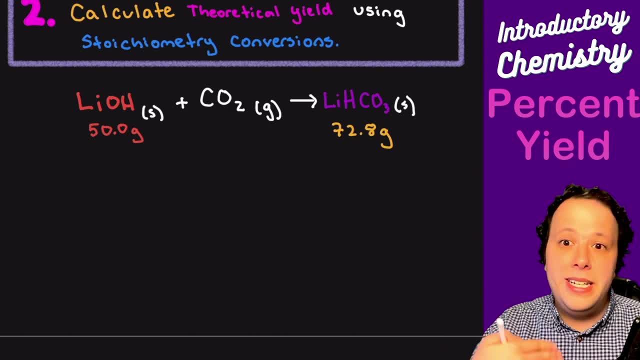 some form or it's what you did in the lab. it has to either be given to you or you did it yourself. there's no. you generally can't calculate it unless you were given the percent yield you have to. usually something has to be given to you. so if we were to do this, we have 50 grams. 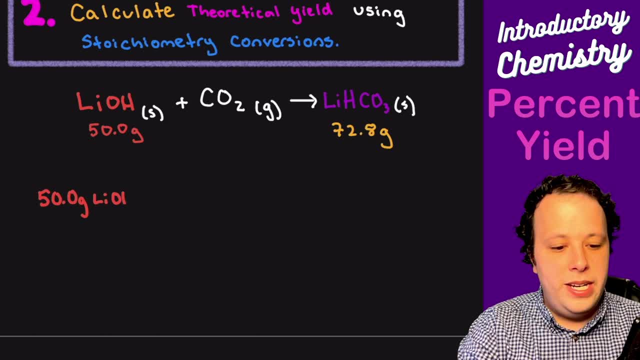 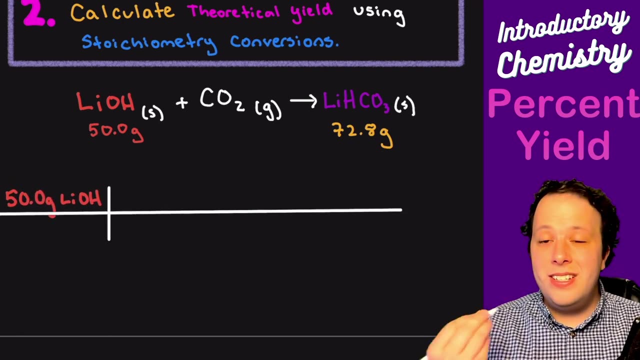 of lithium hydroxide, so l-i-o-h, and we are going to convert this to lithium bicarbonate. so what is our first step? to do that? well, whenever we are given a mass to, our goal is always the mole, so we need to use the molar mass of lithium hydroxide to get there. so what we'll do is we'll use our periodic table. 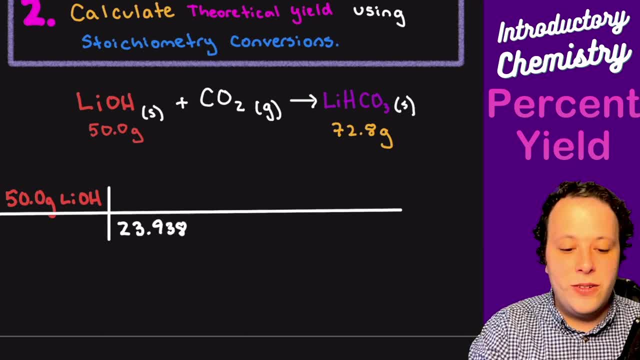 and you'll get 23.938 grams of lithium hydroxide- and if you're watching this, i recommend you check that so you can practice it- and that's equivalent to one mole of lithium hydroxide. now, from there, what we're going to do is use our chemical equation, which we're going to see. it's a one-to-one ratio. 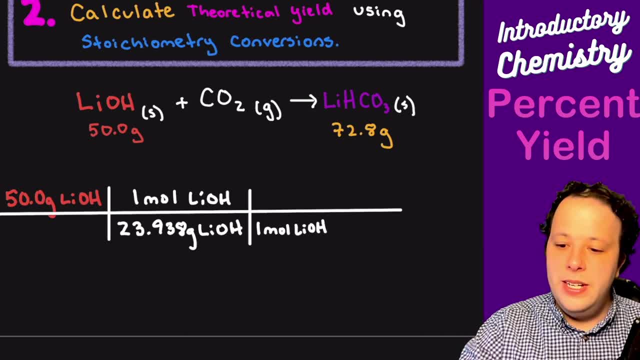 so one mole of l-i-o-h is equivalent to one mole of l-i-h v-o-3. all right, so that's a one-to-one ratio, and let's change the color lithium hydroxide to match the formula too. now, from there we're going. 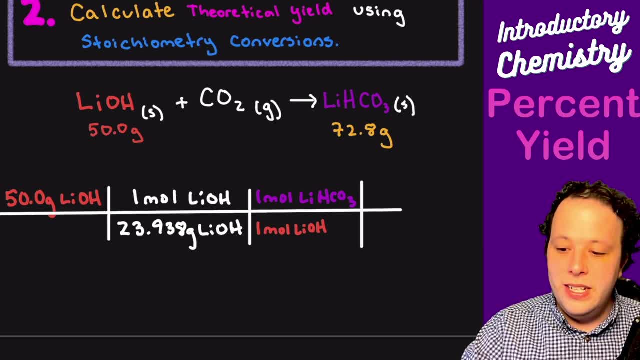 now going to use the molar mass of lithium hydroxide to cancel out the last part. but before we do that, let's just show: our units are all canceling. so grams, canceled grams, and then moles, canceled moles. all right, so our molar mass of lithium hydroxide is going to be one mole. 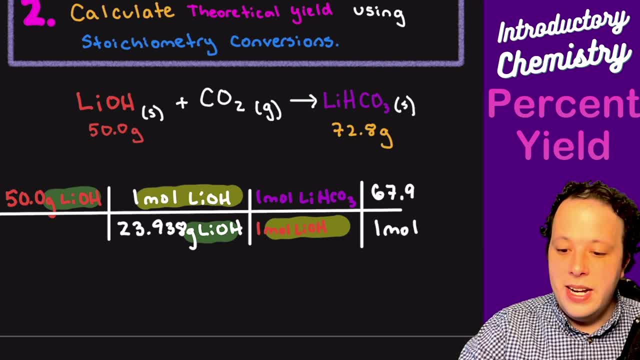 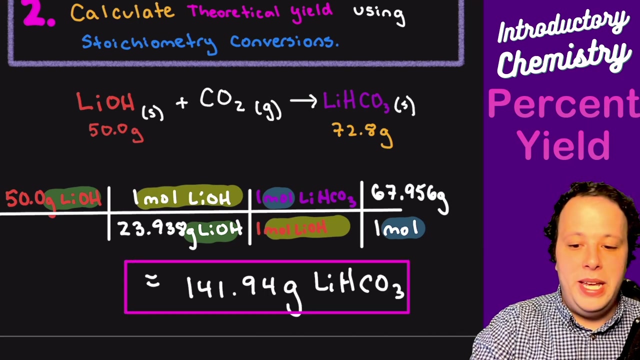 is equivalent to 67.956 grams, and we can see that, hey, these canceled as well. so one mole cancels one mole and what we will get in the end is 141.94 grams of lih co3. so this is your theoretical yield, that we are here and we have labeled in pink. so what do we got to do now? how? 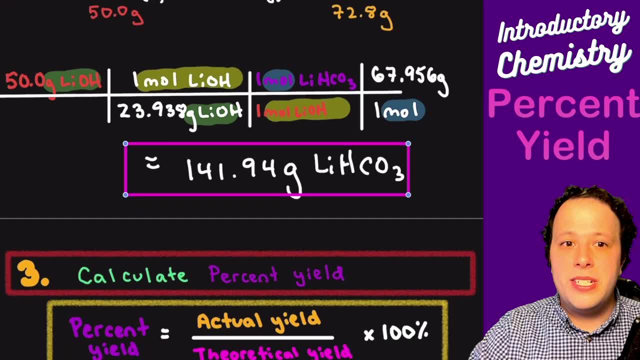 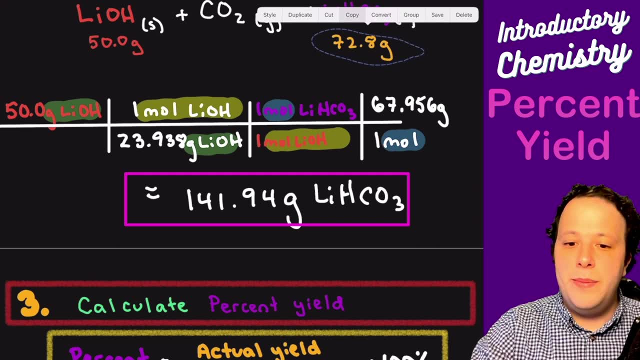 do we figure out the percent yield? well, the whole entire thing with the percent yields. we got to kind of plug it into the formula below. so we were given 72.8 grams is how much we started with. so what we are going to do is we're going to 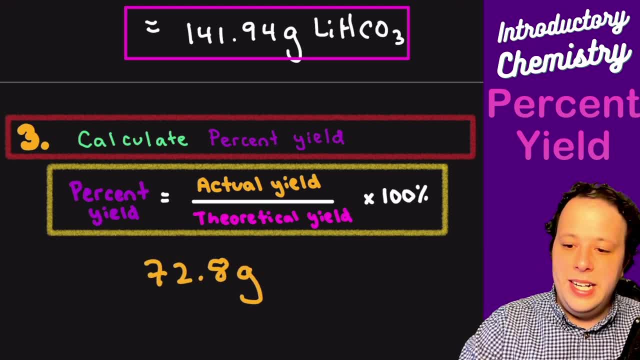 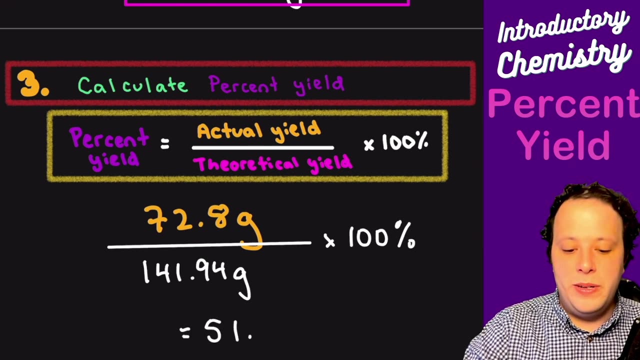 do is essentially take that value and then divide it by our 141.94 grams, and we're going to times that by 100 percent, and what we are going to end up having in the end is about 51.3 percent is our yield in this problem. so which isn't which is pretty good. i know it sounds like a really low. 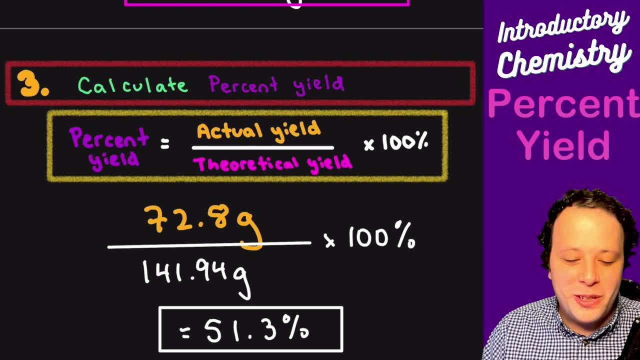 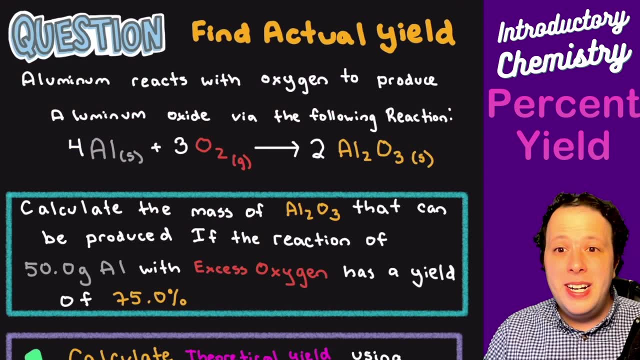 number, but in terms of percent yields this is pretty good for most chemical reactions. you always want to get higher, but it's not bad for a chemical reaction. let's look at another example. so we want to find the actual yield in this problem. so we're going to be working backwards, meaning that aluminum 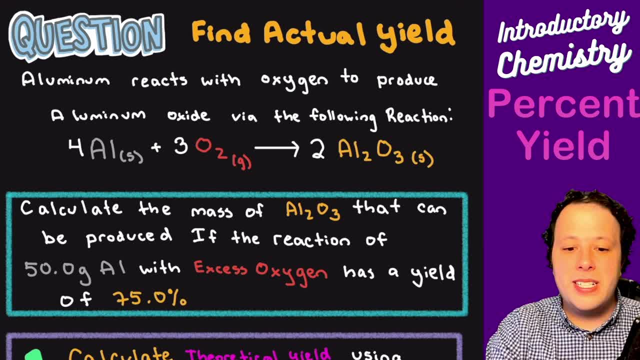 reacts with oxygen to produce aluminum oxide via the following reaction. so we have four aluminum reacting with three oxygen to make two aluminum oxide. so what we are going to do is we're going to calculate the mass of aluminum oxide that can be used to make two aluminum oxide. so we're going to 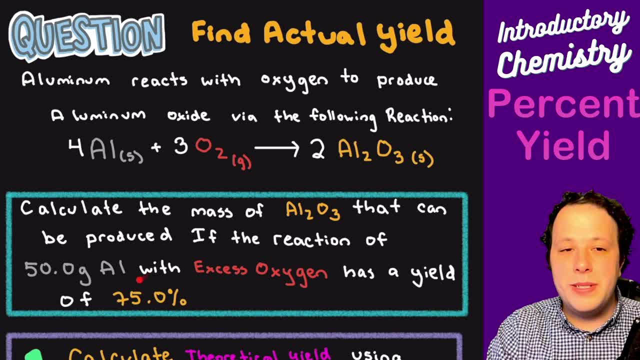 calculate the mass of aluminum oxide that can be produced if the reaction of 50 grams of aluminum with excess oxygen has a yield of 75 percent. so first things first is we need to calculate the theoretical yield, starting with 50 grams of aluminum. so we're going to convert that to 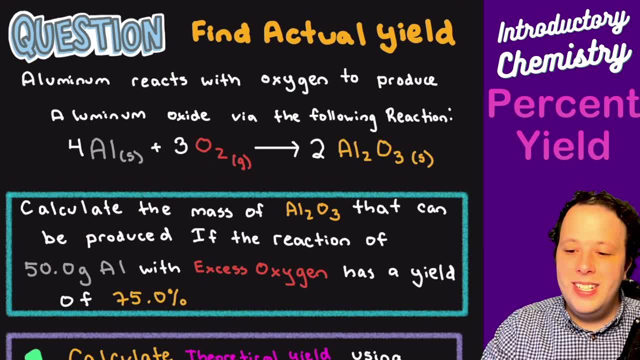 aluminum oxide in this problem. so we got to kind of look through what all the important piece of information is to write. there's a lot of words here, but we only need a few of these more important terms, which was the number of grams of aluminum oxide and the number of grams of oxygen that we need to. 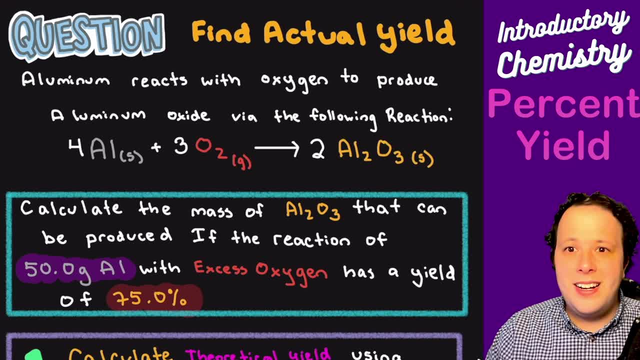 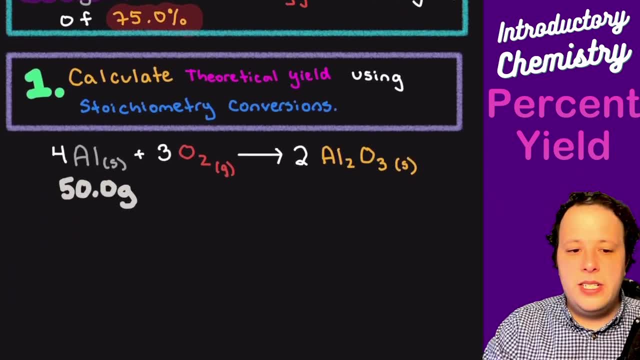 calculate the mass of aluminum oxide to view that value. so we will start with 50 grams of aluminum. excess oxygen means it's not going to run out. and then we have 75 is what our yield is. so we're starting with 50. so what we're going to do is calculate what that theoretical yield is. so we're 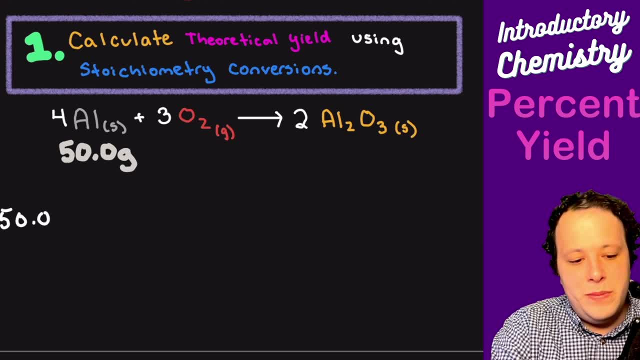 going to start with 50 grams of aluminum and we need to get that two moles. so how do we get a mass to moles? well, we need to use the molar mass to do that. so we're going to use our periodic table to see that, okay, 26.98 grams of aluminum is equivalent to one mole of aluminum. Now we are interested in 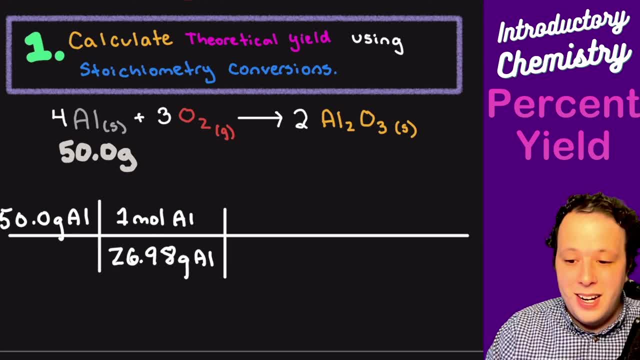 getting to the final product, which is aluminum oxide. So we need to use our molar coefficients to get there. So we see that four moles of aluminum is equivalent to two moles of Al2O3.. Then we are going to use the molar mass of aluminum oxide to get two grams as our final. 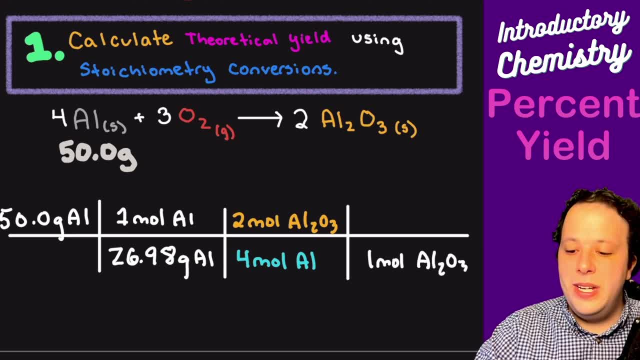 step. So one mole of Al2O3 is equivalent to 101.957 grams Al2O3.. Now, before we continue, we want to double check. did all of our units cancel properly? So we see grams are opposite each other. they canceled, moles canceled. 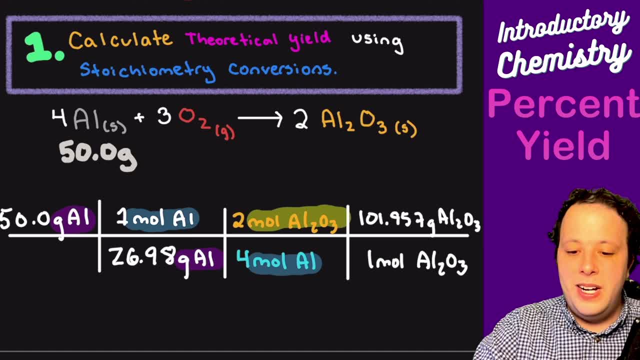 Moles of aluminum, and then moles of aluminum oxide, canceled Moles of aluminum oxide, leaving us only with the grams. So when we solve this, we'll take 50 divided by 26.98 times by 2, divide by 4, then multiply by 101.97, and what we will get for a theoretical yield is about 94.5 grams of Al2O3. 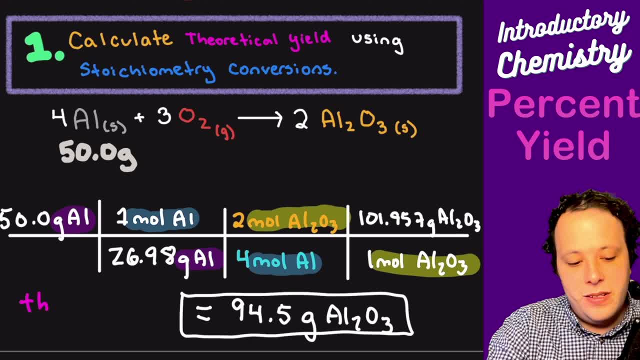 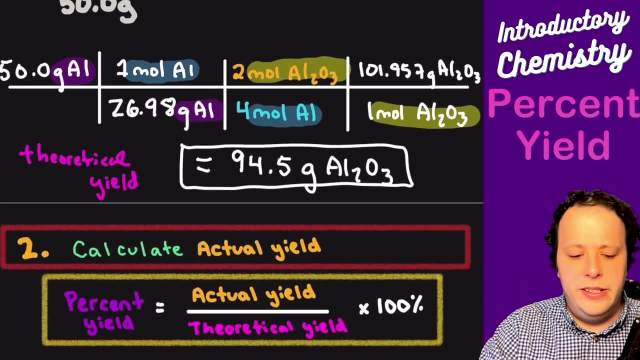 So this is our theoretical yield here, which is how much what we've been doing all along when it comes to stoichiometry. It's nothing new, it's just we're just labeling it a little differently. So calculate the actual yield. How do we do it? Well, the thing is we were given that we had 75. 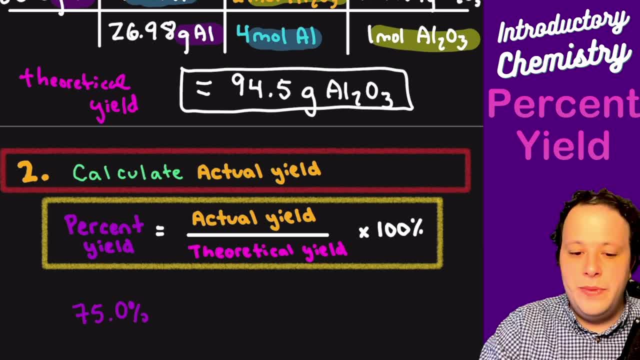 percent, percent yield in the problem. So what we are going to do is we're going to pretty much take the problem and plug in the theoretical yield that we got. So we have our actual yield and then our theoretical was 94.5 grams of Al2O3. 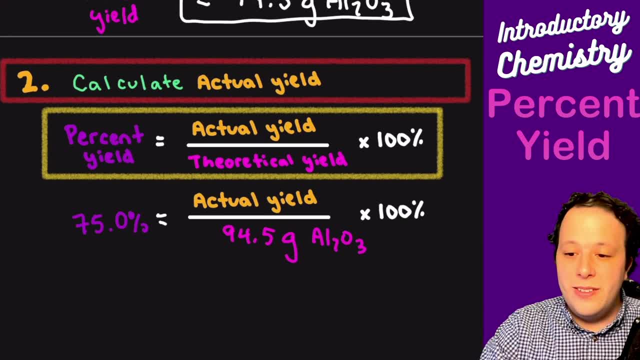 So the first thing we're going to do is we're going to move the 100 percent to the other side, and what we'll quickly get is: all right, 75 divided by 100, we'll get 0.75, and that's going to be equal. 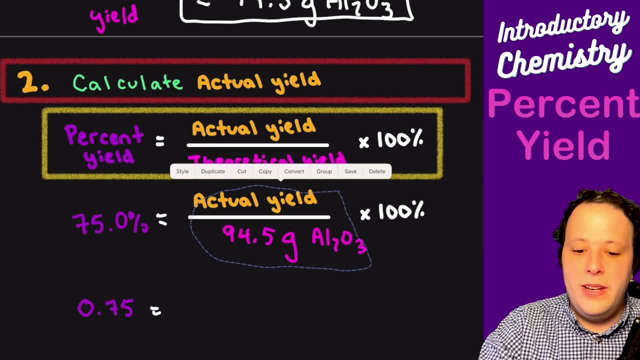 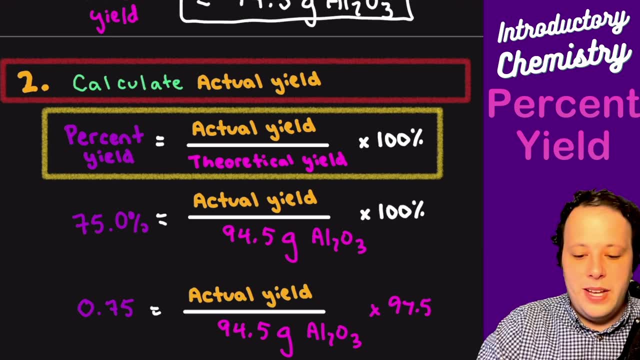 to our actual divided by our theoretical, and then we will multiply both sides by 94.5.. So that will be our actual yield. So we're going to take the actual yield and we're going to plug in the. that way we get that number by itself. 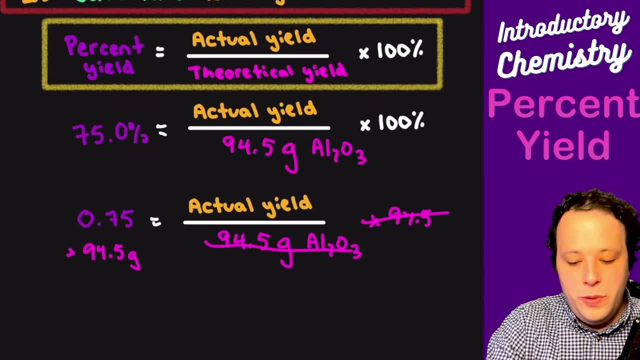 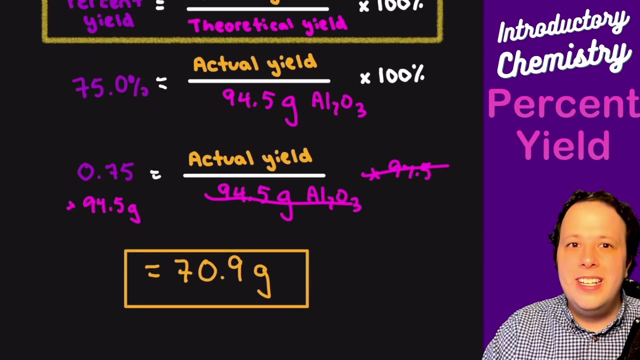 They cancel out, and then what we will have for our actual yield is 70.9 grams. That's how much they actually got in lab. So this is if you had to calculate actual yield, but, as I mentioned before, this has to be a number that's somehow given to you. As you saw, it was given via the percent. 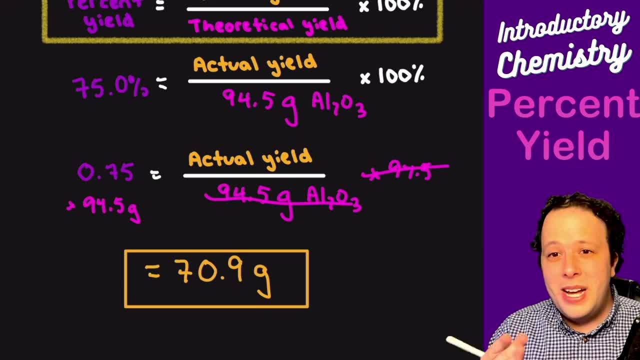 yield. this time It's something that you need to calculate, So we're going to take the actual yield. you have to have to physically do All right. So this has been my video on percent yield and actual yield. This is just another check for yourself to see how you did when you're comparing. 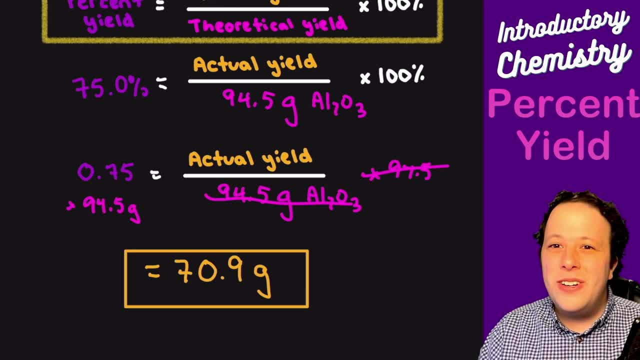 your lab data to what you actually could theoretically get if the reaction went flawlessly All right. So thank you so much for listening. If you need help, please reach out, email me, comment below, ask me in class. I hope that this does help you. If not, I'll see you in the next video. 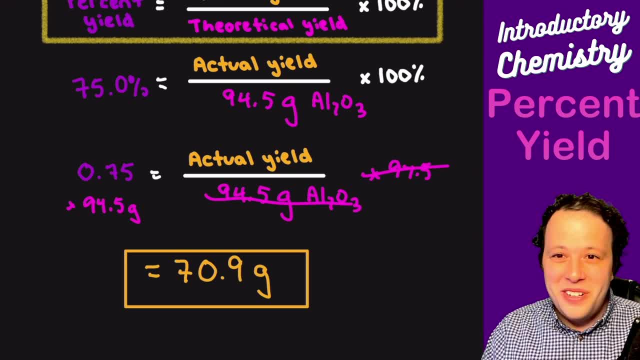 Bye. I'm sorry, But if this is your first time here, please hit that like and subscribe button. Please keep supporting the channel. I really appreciate all of you and I hope you have a wonderful day. All right, I will see you all later. Bye now.